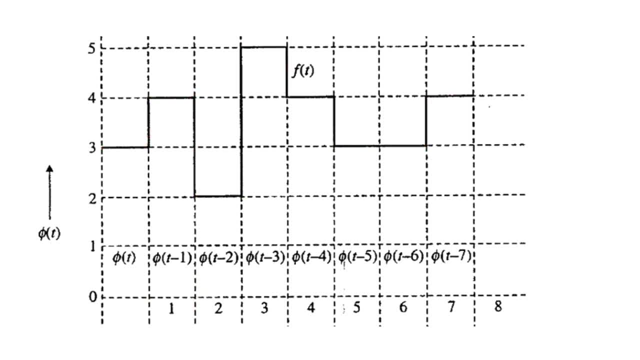 So this much of signal we have discussed in our previous video where upon the functional basis, which are the translated versions of the wavelets. So this is the scaling function, hard scaling function. This is the original hard scaling function representation by phi of t which is having amplitude level 1 or the time interval 0 to 1. here by translating it onto the time axis. 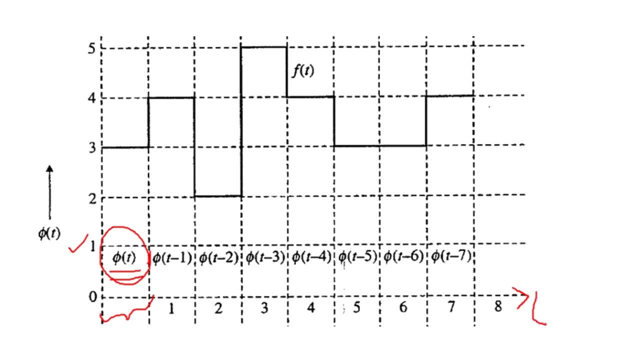 Here it is the time axis. you can denote it by small t as well. We have the translated versions by one unit. If you make translation on the right hand side, it will be phi of t minus 1. translation by two units It will be phi of t minus 2. translation by three units: phi of t minus 3.. So this way we have phi of t minus 4, phi of t minus 5, phi of t minus 6, phi of t minus 7.. 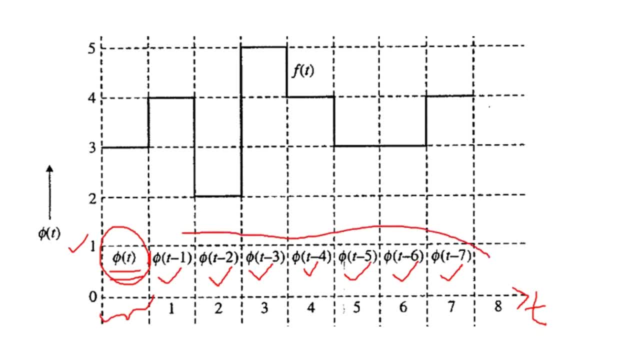 So when we use these functional bases to be the set here we have called it to be the functional space defined as capital E0 here. So for every such a functional base here, which is a translated version of The original hard scaling function, we have to make further scaling to achieve the particular amplitude level. 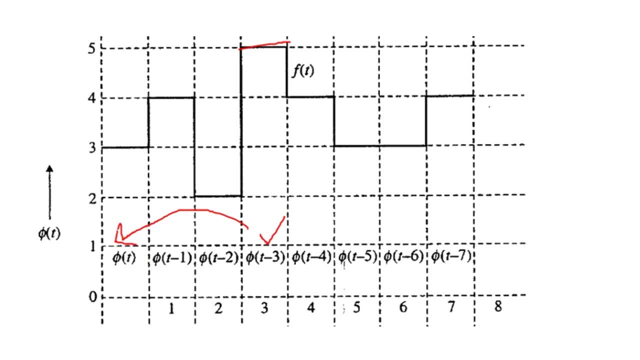 So for this one it should be scaling by phi, so we can have the representation of this amplitude level as phi times phi of t minus 3.. So for this amplitude level we can have the representation three times, as this is the amplitude 3- here it was the earlier phi- 3 times phi of t minus 5.. 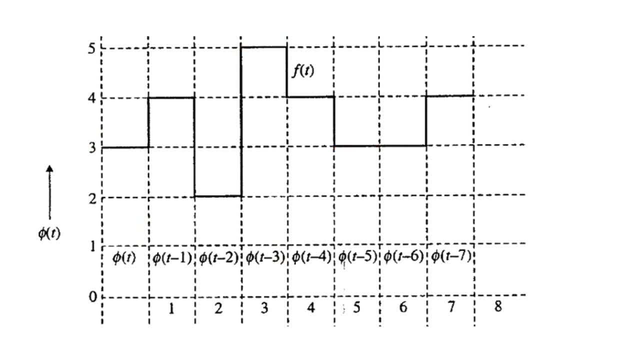 So this way, if we have the Representation and if we are successful to correctly convey the information as we have graphically illustrated here, we can call that this is the representation into the functional space capital V0 here. Next to that we had seen one more illustration where it was another random kind of the signal where the amplitude levels into the unit intervals were not constant. 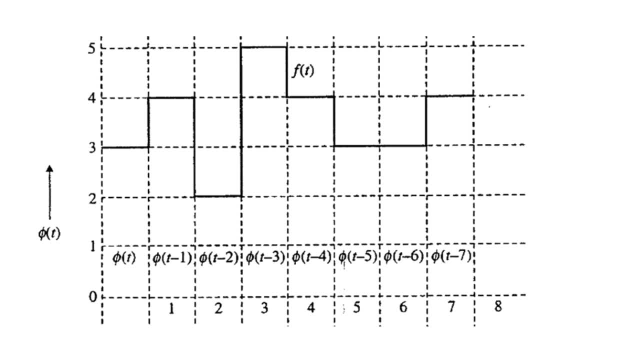 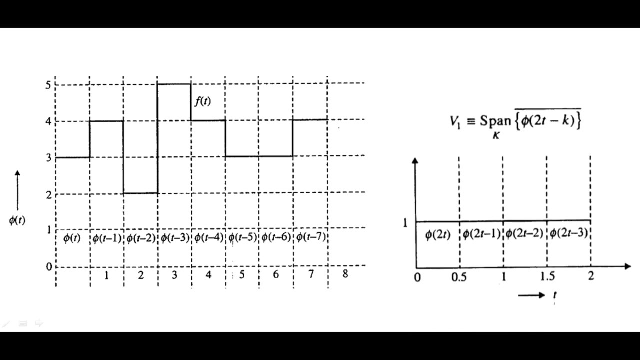 They were either linearly varying or randomly varying. That created the need to have more finer convergence of these functional bases here. That is why in general we have Vj as the functional space. The next functional space after phi 0 was obtained by reducing the time interval for the base functions by half here. 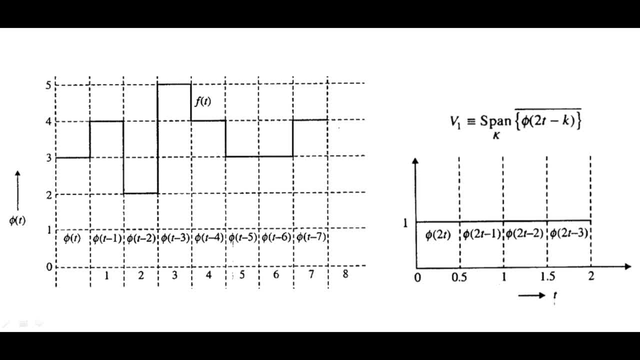 So it was made to the half. So reduction factor was 2 here, So that time we had obtained The V1. As the functional space, And this was the mathematical expression to denote the same here where the functional basis you see phi of 2t, phi of 2t minus 1, where the 2 to be constituted for phi of t only. 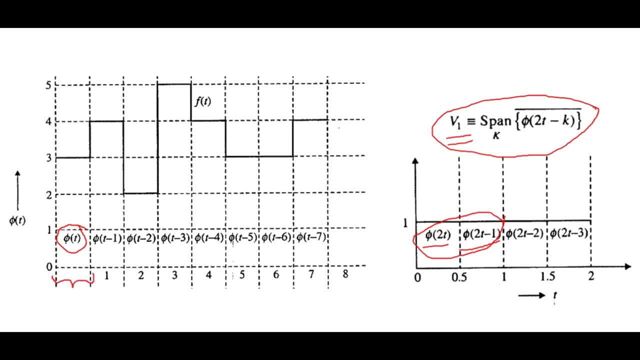 So this phi of t, which spanned for 0 to 1, is represented by the 2 here. So this is 0 to 1.. We have make it half 0 to 0.5 and 0.5 to 1 here. 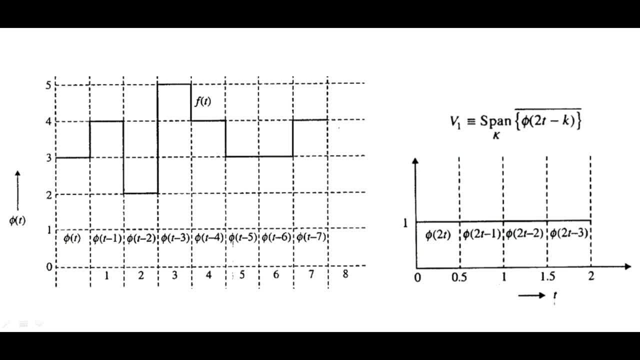 So this is the another functional space we can call. So after V0, we have V1 here. So let us have the representation of the signal that we have shown with the help of the solid line, starting at the amplitude level 3 and ending at the amplitude level 4 here. 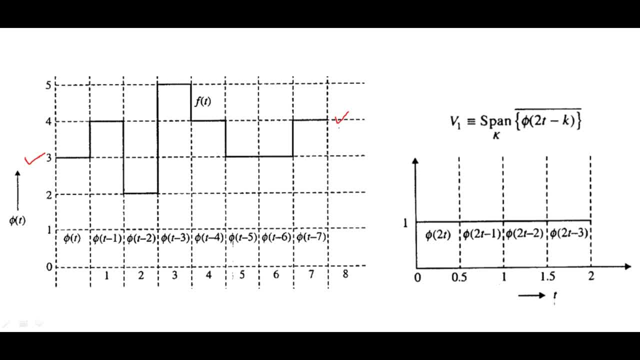 By using the functional space V0. That is making the use of Base functions from this set and then from V0, which is making the use of the base functions from this set here. So on the next slide you see the signal denoted by f of t here. 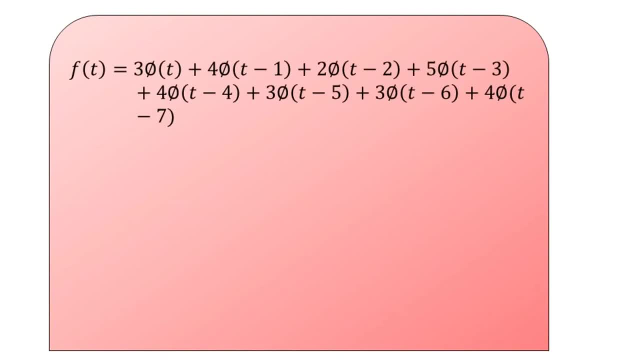 So f of t we represent by the use of V0, as the functional space f of t is equal to 3 times phi of t added by 4 times phi of t minus 1.. Further Added by 2 times phi of t minus 2, added by 5 times t minus 3 phi of t minus 3, further added by 4 times phi of t minus 4.. 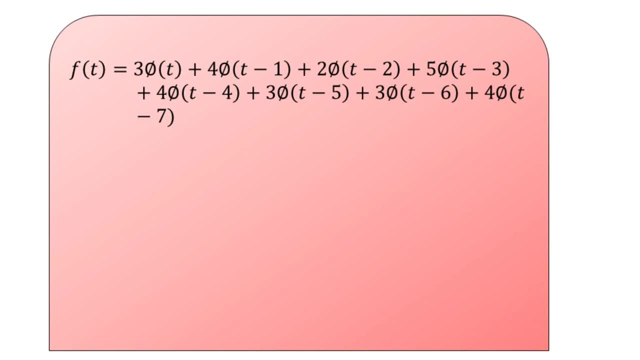 Next to that we add it with 3 times phi of t minus 5, plus 3 times phi of t minus 6, and at last the addition is with 4 times phi of t minus 7.. So this is the functional representation by V0.. 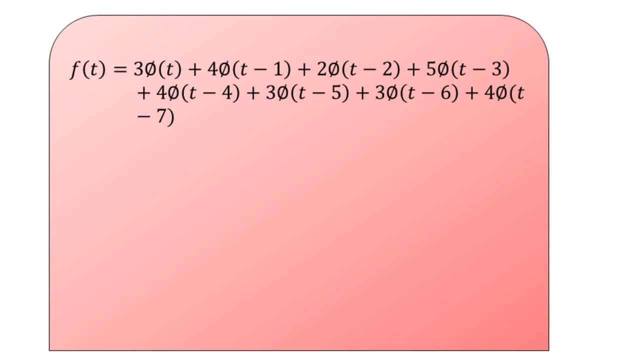 If we make the use of functional space V1, we get this representation. See, this is the generalized representation for the signal that we illustrated earlier. So you see these two terms: 3 times phi of 2t added by 3 times phi of 2t minus 1.. 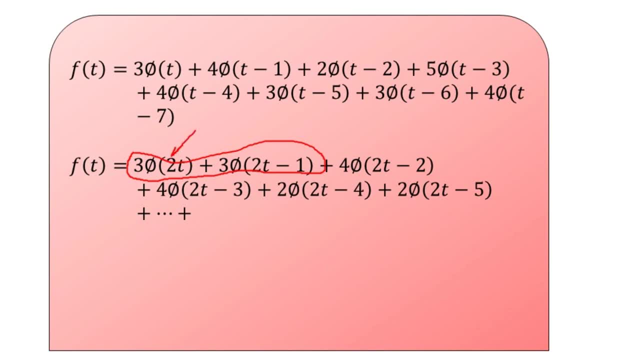 So we have the two translated versions after reducing the time interval of the correlation. So we have the two translated versions after reducing the time interval of the correlation And we have the single scaling function by factor 2 here And both are having V scaling by the same factor. as for that per起來 span, we need the amplitude cable equal to 3 here. 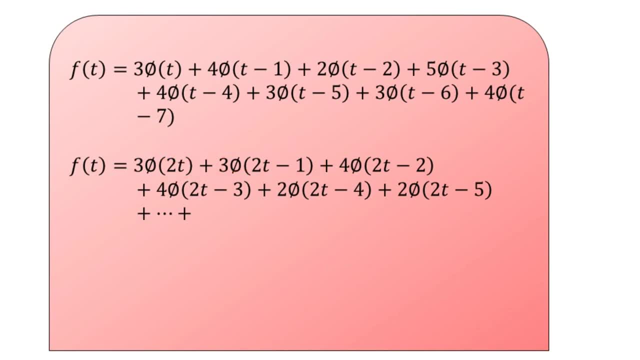 So for every term in the earlier representation we have two terms in the new representation. So for 4 times phi of t minus 1 we have 4 times phi of 2t minus 2. Added by 4 times phi of 2t minus 1.. 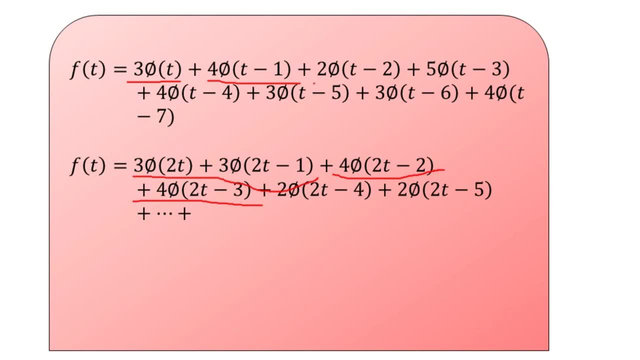 So we have the same 2t minus 3. 2 times phi of t minus 2 will be constituting the two terms as like here. you see the same scaling factor, 2 multiplied to first of all phi of 2t minus 4 and then phi of 2t minus. 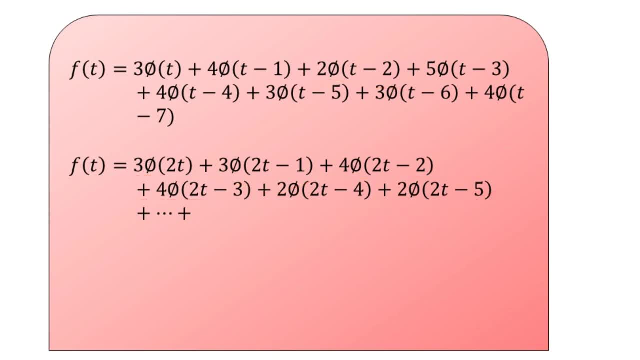 5 here. so these two representations are conveying the same information but by the use of different functional spaces that we have defined as capital V0 and then capital V1 here. so now to see the two terms for every term of the earlier representation. in general we can say that capital V0- functional. 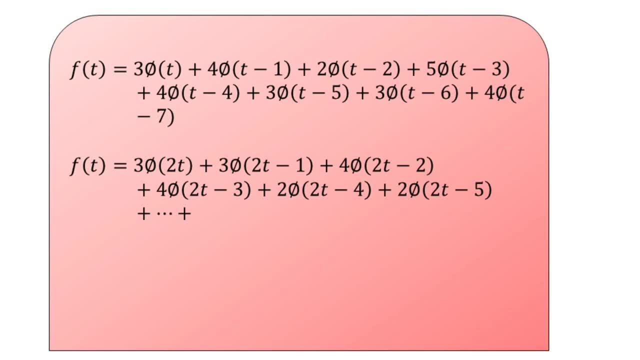 space is contained into the capital V1 functional space, or in another words we can say V0 is a subset of V1.. You see, capital V1, the functional space, is more finer functional space than that of the V0 and it can contain all the signals into the V0 here. Here we have V1. 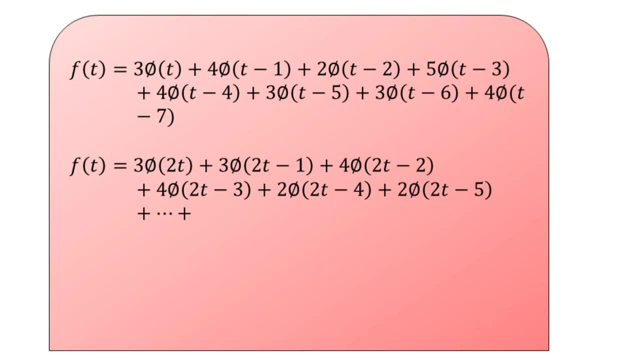 to be the bigger space than that of the V0 here. Why is it possible? Because the basis of V0 itself can be represented using the basis of V2.. We have just now seen that for every functional base, as it was 3 times phi of t, we have substituted it by 3 times phi. 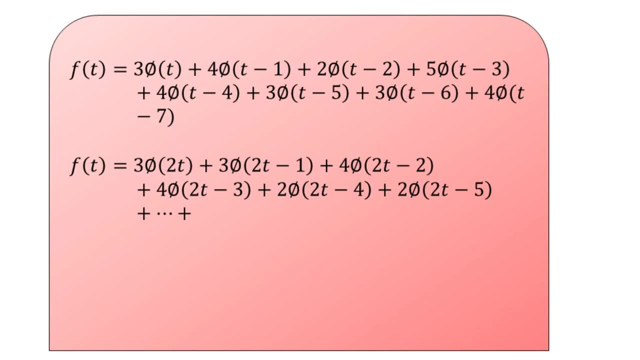 of 2t plus 3 times phi of 2t minus 1.. We have substituted 4 times phi of t minus 1 by 4 times phi of 2t minus 2, added by 4 times phi of 2t minus 3, and so on here. 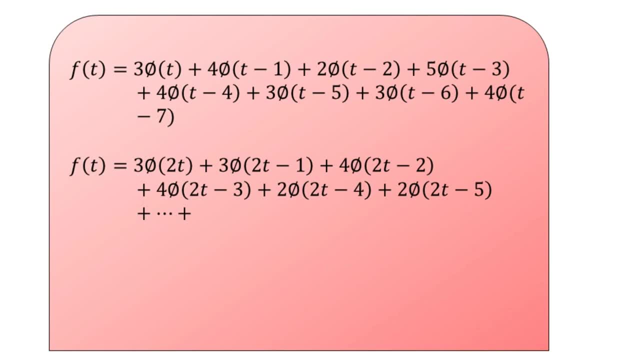 So now here, for example, let us have: phi of t is equal to as represented here, and phi of t minus 1 here. So on the left hand side we have the functional basis from V0 and from the right hand side we have the functional basis from the capital V1 here See the relationship. 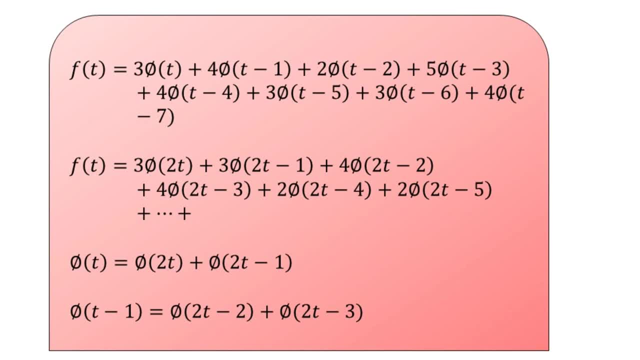 between the functional basis from the two functional spaces V0 and V2.. We can call the last two formulas to be the scaling relations, or most popularly it is also known by the term refinement relation, or you can also call it to be the dilation equation here. So as just now we have concluded that V0 is a subset of V1. Similarly, we can 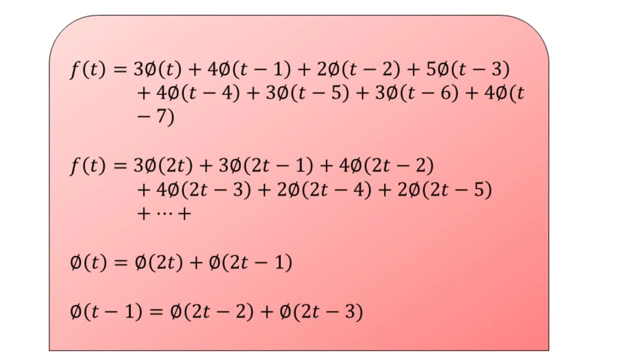 also prove that V1 is a subset of V2.. So, that is, any signal in V1 can be represented using the basis of V2. and again, this is possible because any basis of V1 can be represented using the basis of V2.. We shall show you phi. 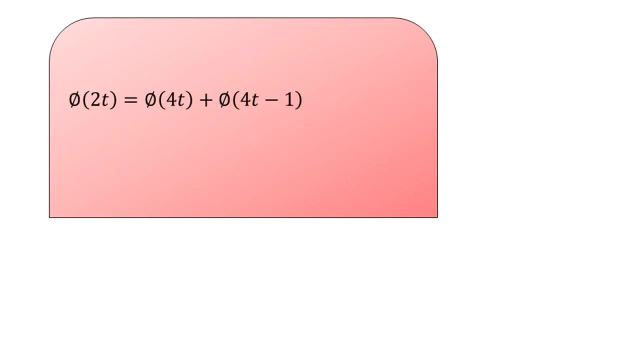 of 2t can be represented as phi of 4t, added by phi of 4t minus 1 here. So for phi of 4t you will have the time interval zero error in of time interval. Know when pi of 4t is. 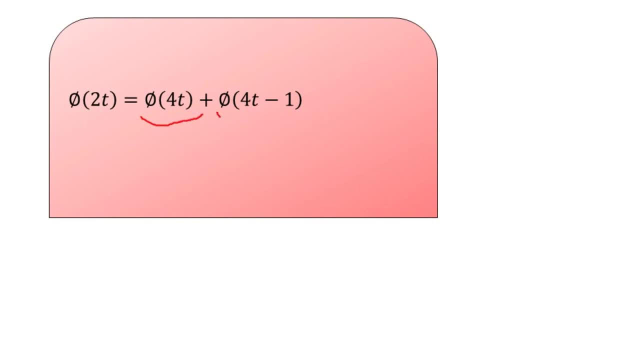 to 0.25 here. you will have 0.25 to 0.5 here. so originally i of 2t is planning for 0 to 0.5, only half of the interval as compared to the original r scaling function here. so this way we can have: 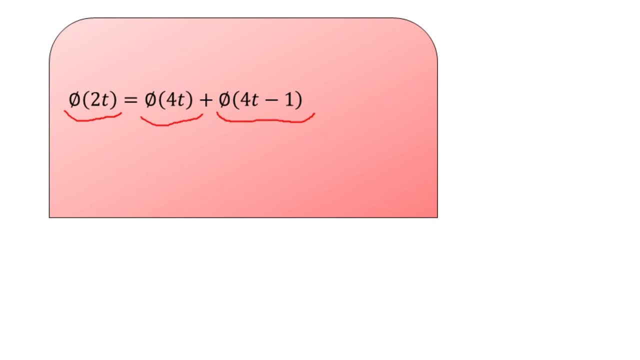 the reductions and reductions to obtain more and more finer versions of the hard scaling functions here and we have also seen the relationship as we go on to obtain more and more final resolutions into these scaling function versions of the r wavelength here. so in general the relationship between them we can represent like this: so you start at v0, so you can see v0 is a subset of v1. 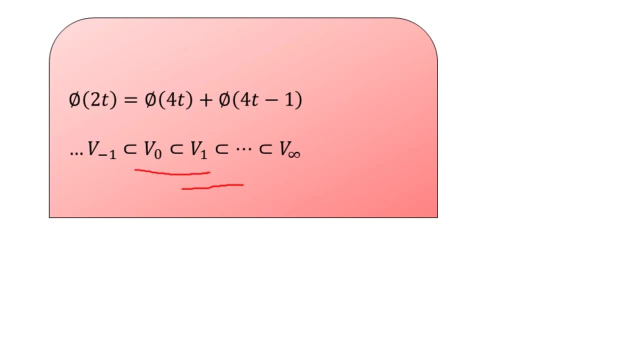 v1 is subset of v2 and in this way you can go up to v- infinity. this is the theoretical writing here, but practically we will have a certain real number in place of infinity. where we will be stopping here. in the left hand side we can have: 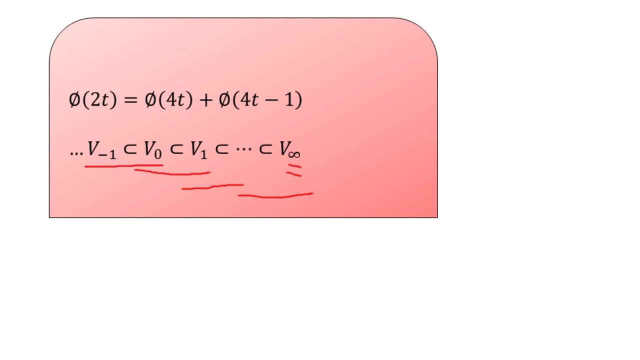 v minus 1 to be the subset of v0. so for v0 the scaling function was spanning for 0 to 1, with the constant amplitude level equal to 1. in the v minus 1, of course, the constant amplitude is equal to 1 and in case of v1 the amplitude of often is equal to 0. so the amplitude, of course, the constant amplitude of the constant amplitude. 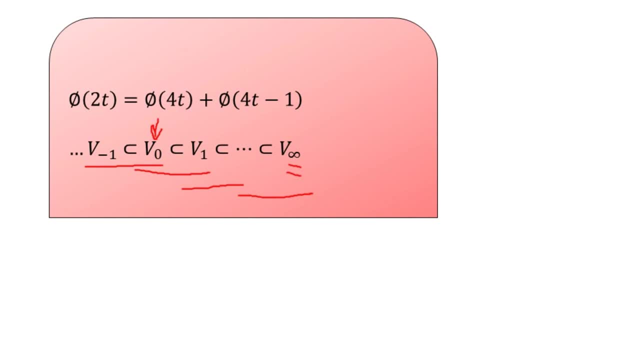 to level will be equal to 1, what we can score scale to any value by just multiplying it. but it will be spanning, for let us say for example, in this particular case 0 to 2 and then onwards 2 to 4. so this way we can have more combinations here. so what the relation is important here, what you 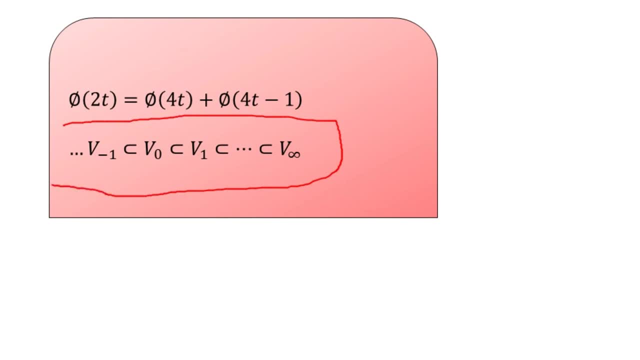 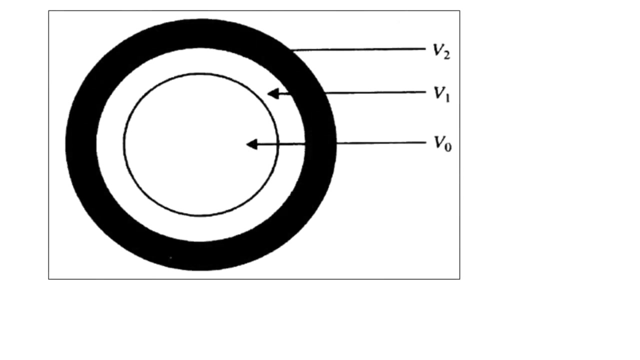 can also outline here, can also be illustrated with the help of the diagram here, which is more prominently obtained and known as the nested spaces diagram here. so I will show you the nested spaces diagram here. you see, V 0 is the inner circle where this V 0 is a part of V 1 also, and 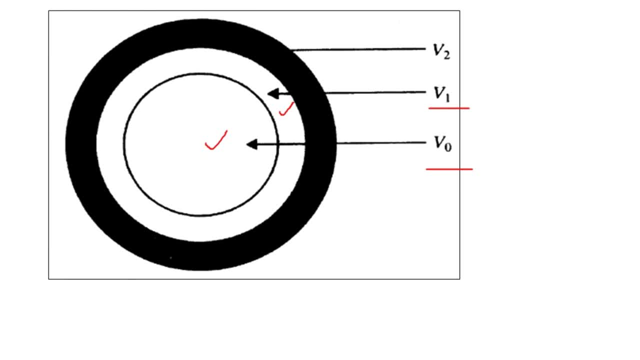 this V 1 is also a part of V 2. here you see, and this way we can go for any positive numbers or the negative numbers inside this V 0, what we can call the nested spaces. for the nested spaces, the very important thing to note down, the refinement, the relation, the relationship.